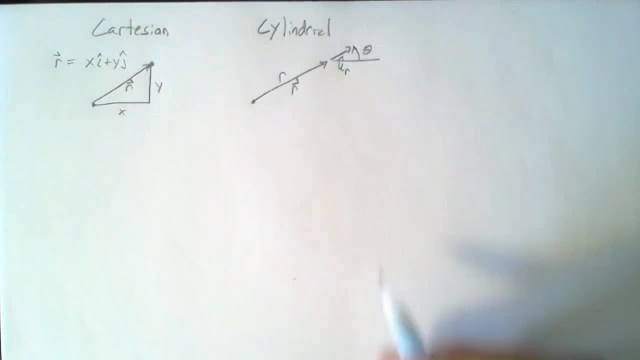 this direction is going to be defined by a theta. Okay, then, finally, we're going to have a path-based representation. Now, this one's a little tricky: You're required to know what the entire path of the particle is going to be. 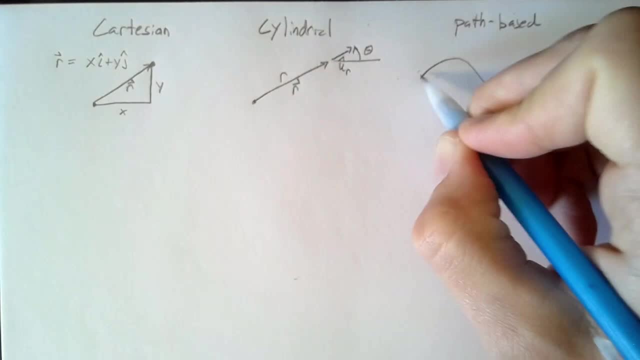 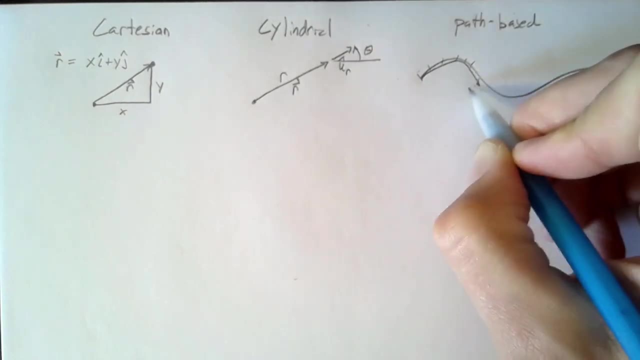 Once we have all of this information, then we're just going to chop this up into sections and then the position along this path is going to be encoded as theta, So we're going to call this: s: this distance At any position s the curve of our path is going to tell us our unit vectors. 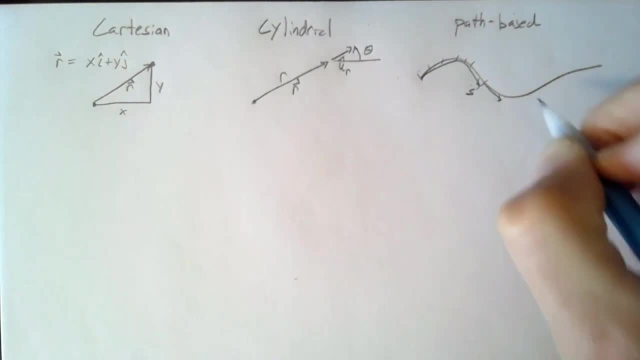 And so at this point we would have a unit vector tangent to the line That's simply u, t, And some unit vector normal to that line which we're going to call u, n. And if we were working in 3D, 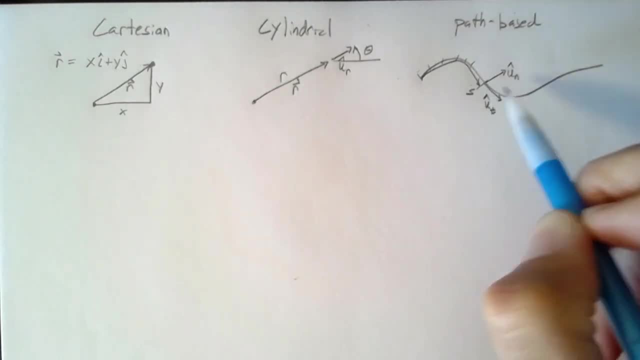 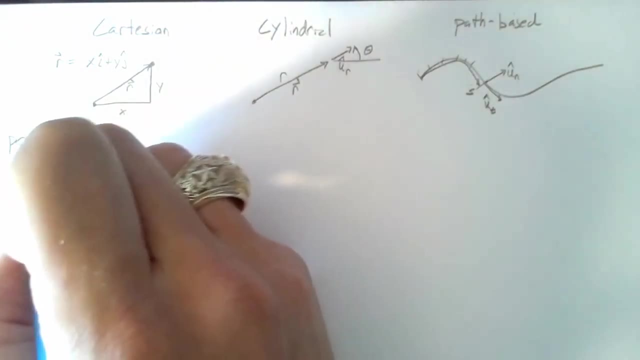 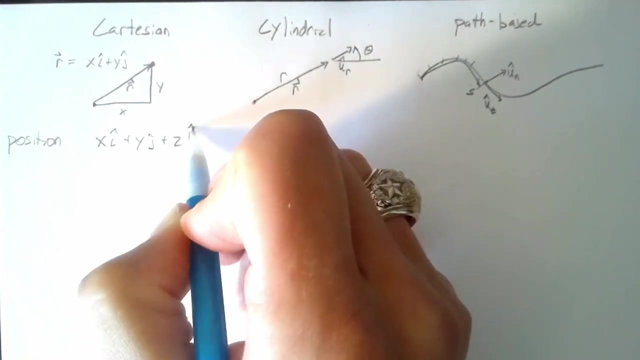 then we would have a binormal direction which is normal to both of these. Okay, so let's write this out For position. we're going to have x, i plus y, j plus z, k, These three unit vectors multiplied by some values. 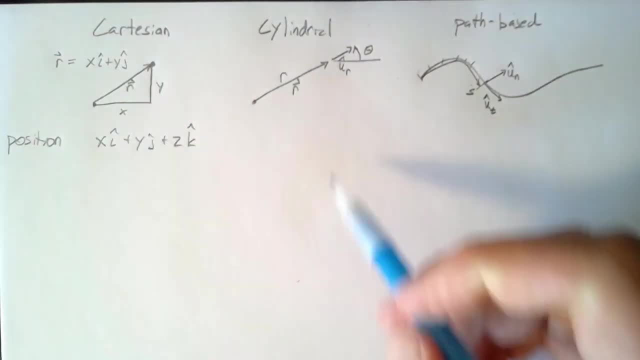 representing how far we are in the x, y and z direction. Here, most of the information is actually encoded in this unit vector, And so all we need to know is the distance multiplied by that unit vector. Finally, for path-based, 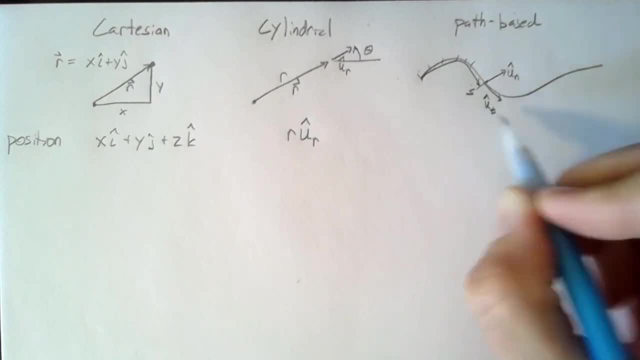 this is actually not easy to encode, So I'm just going to call this s. So this s is the distance along this line. We need a lot more information because we need to know exactly what this line looks like, But, regardless, we're just going to call this s for now. 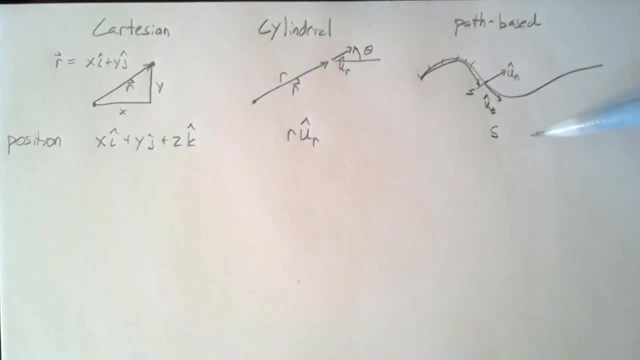 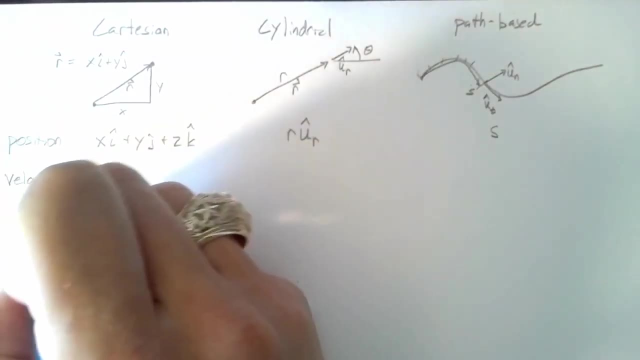 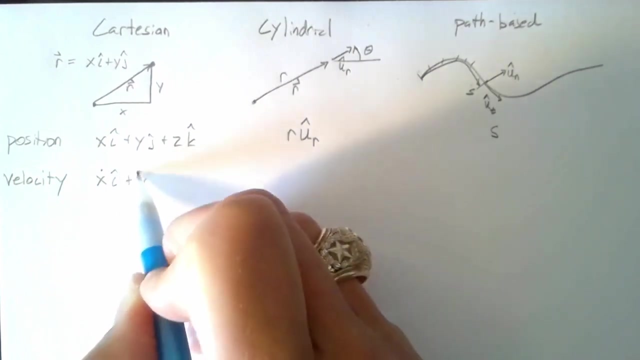 Okay, So that's position. We want to move through and get velocity and acceleration. These are kind of the building blocks of dynamics. So our velocity for Cartesian coordinates is going to be x dot i plus y dot j plus z dot k. So if we have some formula for our position, 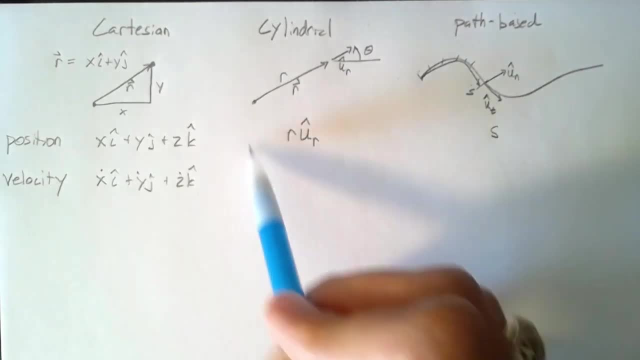 we're going to take the time derivative of each of these pieces and just use that as our velocity. It's all very straightforward. We can ignore the j and the k whenever we're talking about the i. We're just interested in using one piece at a time. 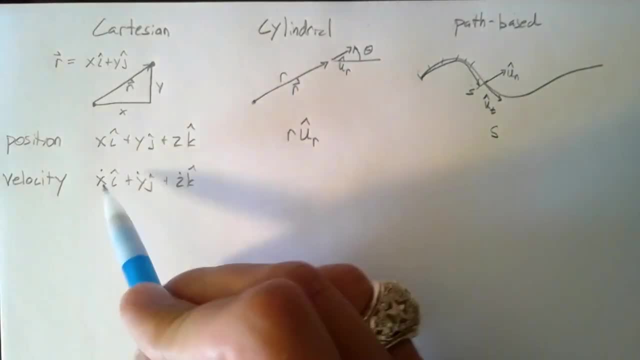 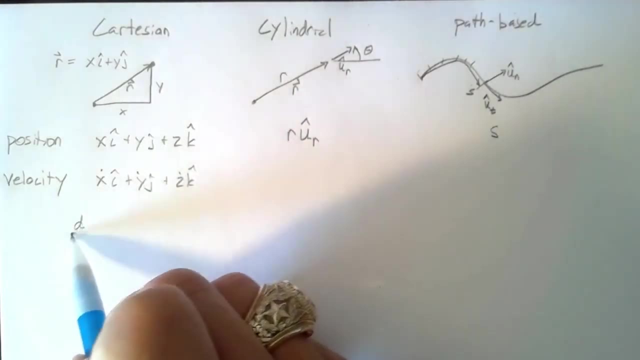 And we just work through that and take the time derivative. This dot, by the way, is how I'm saying the time derivative. If I were to actually use the d by dt over and over again, I'd just be wasting everyone's time. 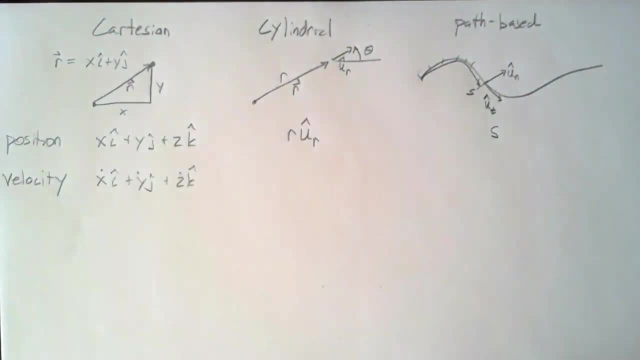 So don't worry about that. Okay, Things get a little tricky whenever we get to this point. Things get a little tricky whenever we get to cylindrical coordinates. The reason for this is not only can this distance change the distance from the origin. 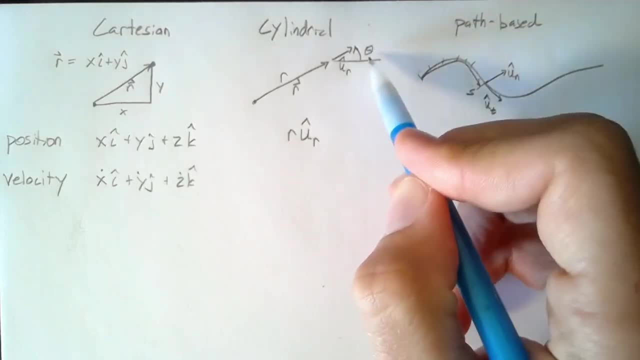 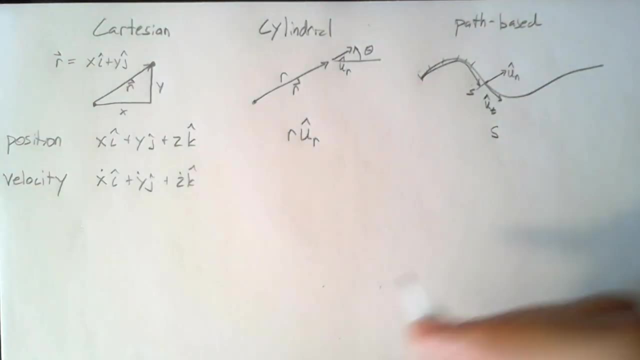 but our theta can change as well, And the reason that that's important is because this u? r can change in time. So the trick here is that we need to define how this u r is changing. So if we wanted to take the time, derivative. 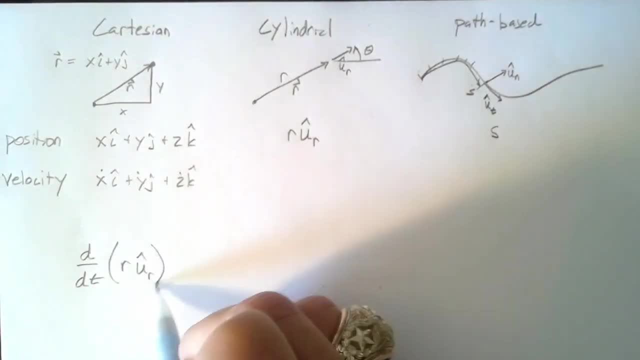 of r times the unit vector. all we have to do is use the product rule. We're going to take the time derivative of the first factor here, so d by dt of r, multiplied by the non-derived, u hat r And we're going to add that to the r without taking the derivative. 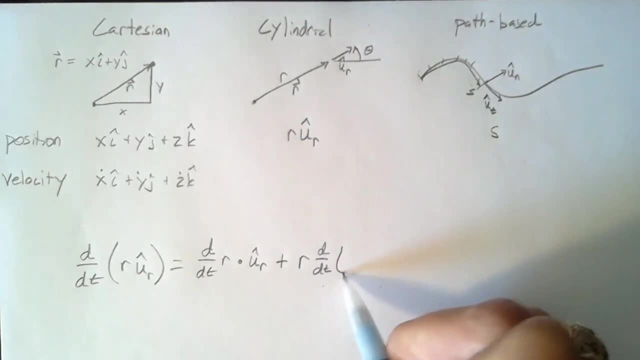 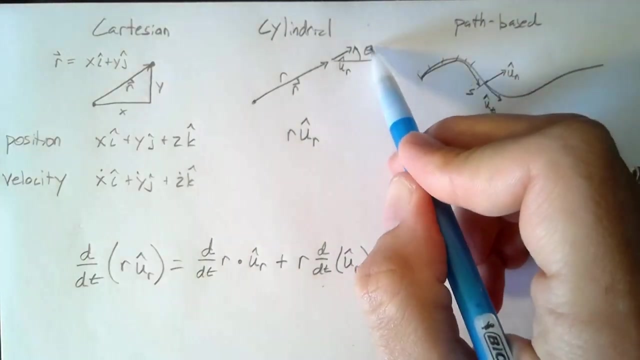 multiplied by the time derivative of u hat r. So now the trick is: how do we actually figure out what the time derivative of this unit vector is? Well, the direction of this unit vector is actually defined by this theta. So if we have some theta, 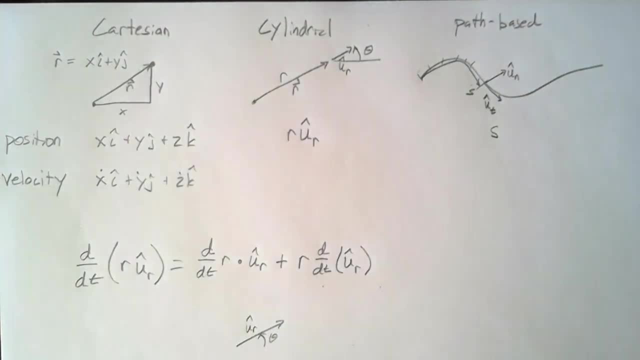 and that defines our u? r and our theta is changing. that's the only way that u? r can change. we have to have some theta dot as well, some time, derivative of theta. So if we have some change of theta, what we're going to end up with is 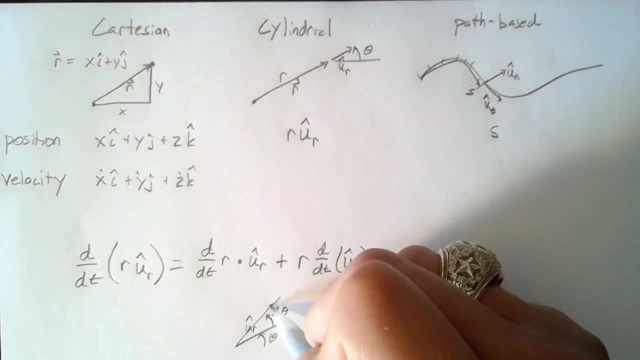 a change of this u r in this direction. Now, what direction are we actually talking about here? Well, we haven't defined it up here. We're going to call this value. we know that a change is based on theta dot and we know the direction is normal to the radial direction. 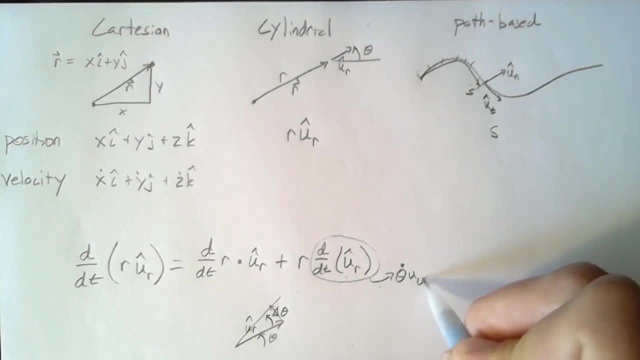 So this is going to change in the u theta direction, And so we're just defining this unit vector to be normal to our radial vector. Okay, so what does this mean? Now we can write our velocity in cylindrical terms. We get r dot. 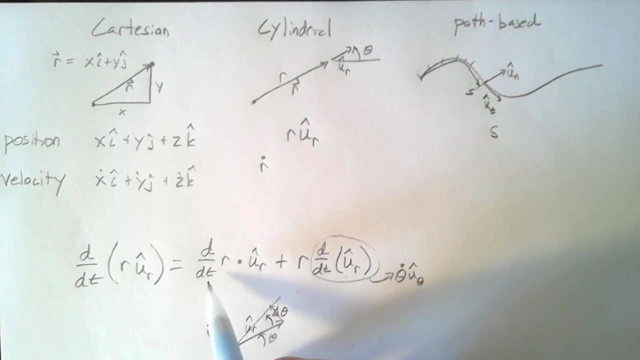 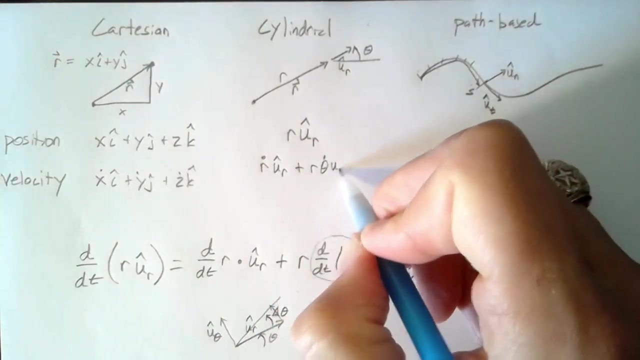 because I said that I'm going to use the dot as the d by dt Multiplied by u hat, r, And we're going to add that to the other component that we got from this product rule, which is r multiplied by theta, dot u, theta. 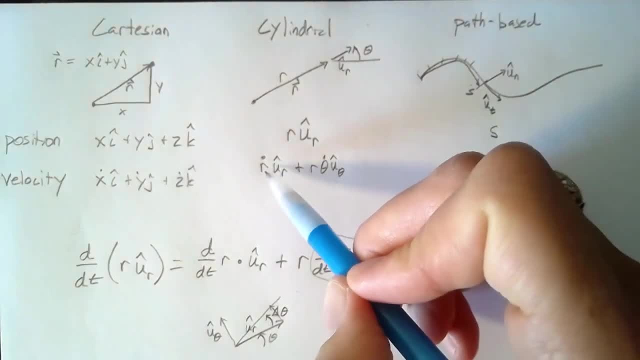 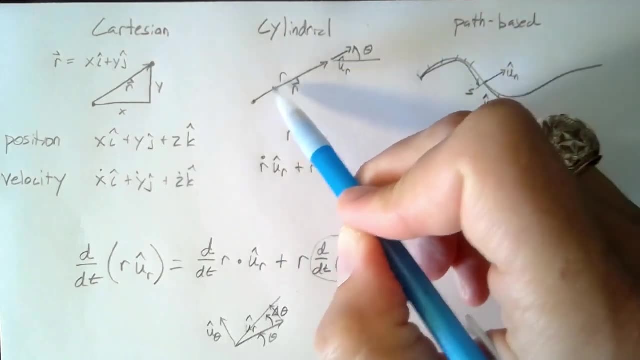 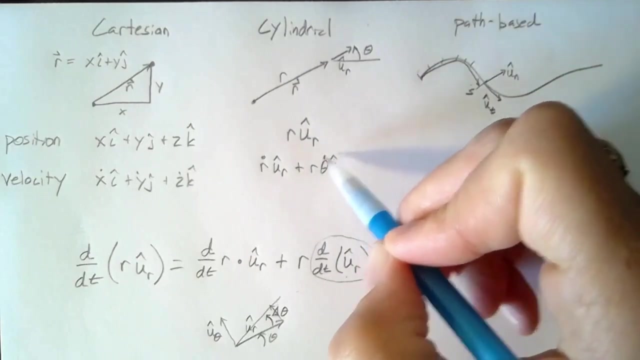 So what is this saying intuitively? Well, the velocity is based on the change in r. So if we ignore this part, then we can have some velocity by our distance extending, increasing our distance in the u? r direction. Okay, we can also have some velocity. 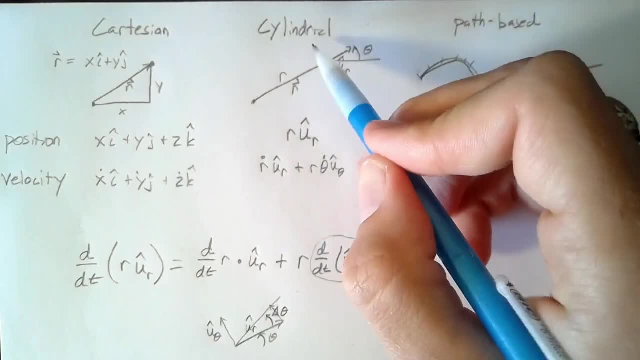 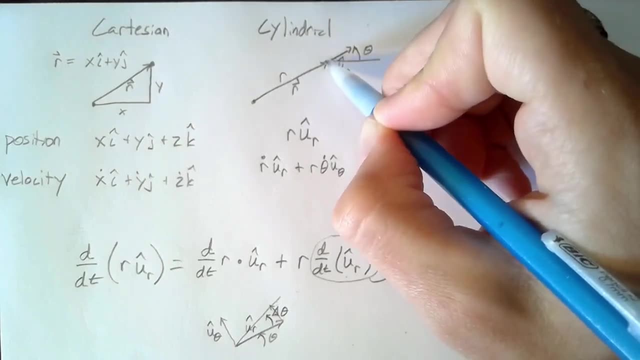 a change in position because our theta is changing. Now, if our theta is increasing, that means that we're moving in this direction. Our u theta is in this direction. So this component is defined by our distance multiplied by the change in angle. 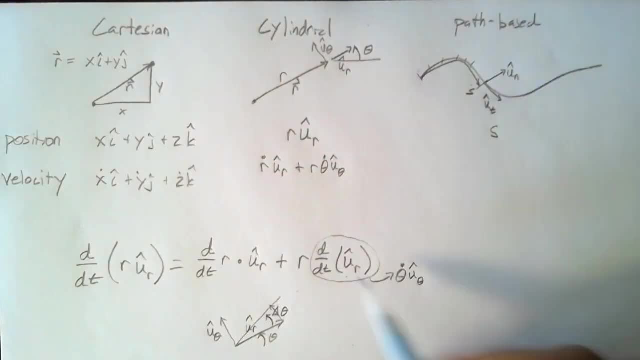 in the u theta direction. Now that we've gotten all that math out of the way, we can move on to the path based, which is actually very easy, Because our tangent vector is defined as the way that our particle is moving. we can actually say that we have some velocity. 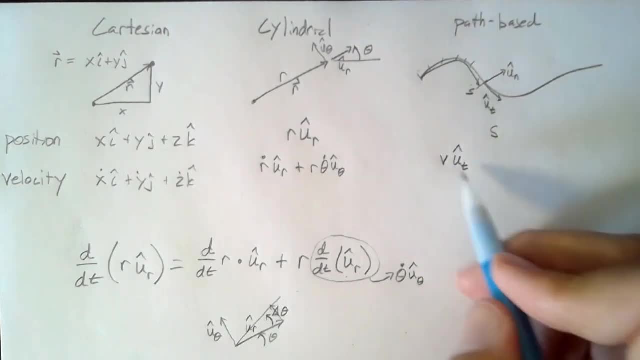 in the u? t direction. So this is the tangent direction And I'm going to define our velocity as s dot. So we have some time derivative s, which defines our velocity, And our velocity by definition. we don't have to do any math to prove it. 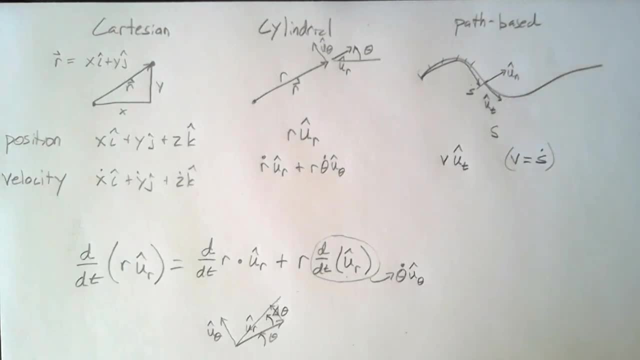 our velocity is in the tangent direction. Okay, one last thing to work through, that is the acceleration Cartesian. very, very simple Again, all we're doing: x double dot in the i direction, y double dot in the j direction. 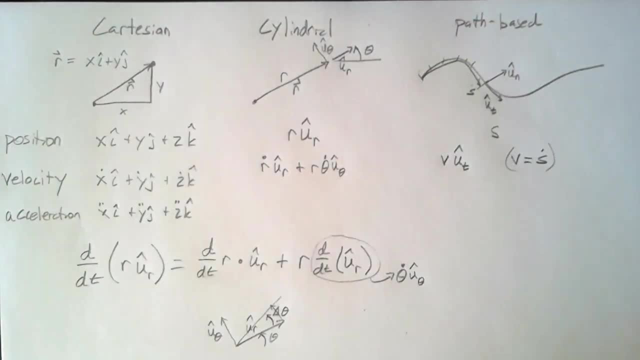 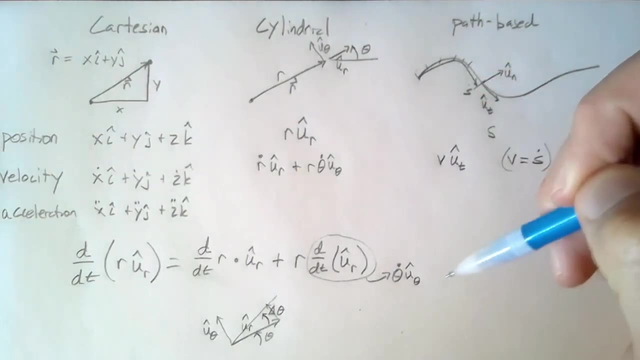 and z double dot in the k direction. Nothing else to worry about. When we get to cylindrical, things get a lot more complicated. So we're going to go back down here to our scratch pad and derive this again just using the product rule. 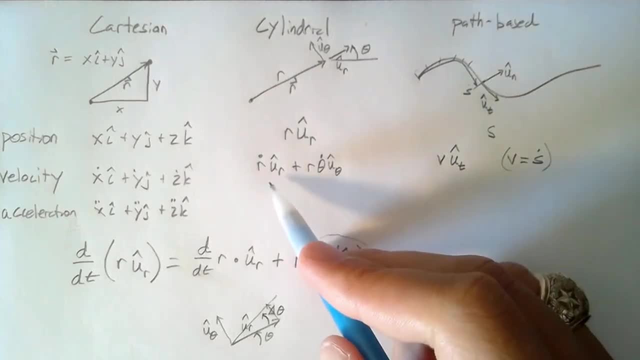 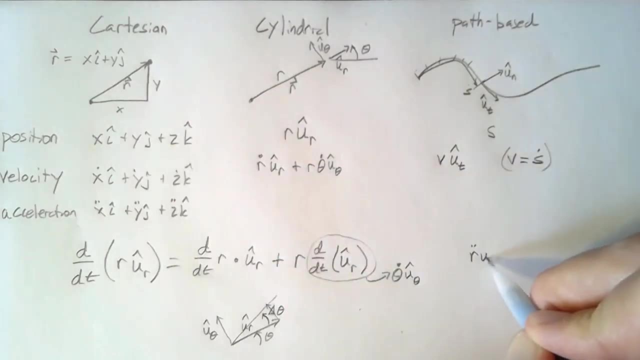 That's all we need. So the product rule for this first term is going to be r, double dot, again deriving the first half, leaving the second half the same, And then we add the derivative of u, r, which we said is theta dot, u, theta. 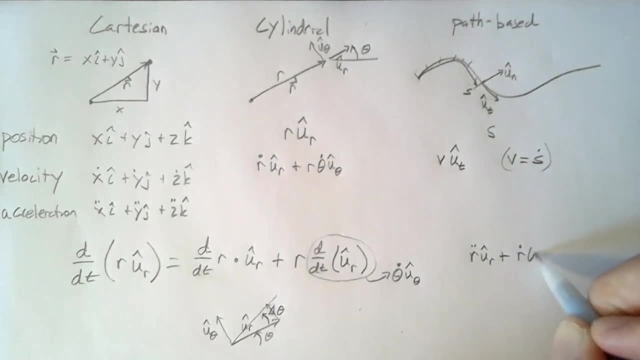 multiplied by r dot, So r dot theta, dot u theta. Okay, now we can read this. Move on to our second term. So we're going to have r dot theta, dot u theta. Then we have to add in the derivative of this guy. 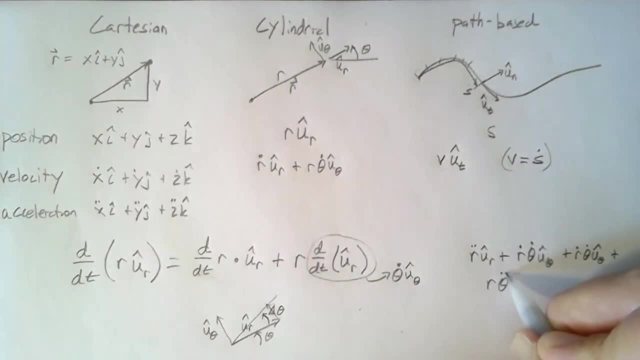 multiplied by the other two. So we're going to have r theta double dot, u theta. And then, finally, we take the derivative of u theta. This is going to be r theta dot. and then we have to think a little bit again about what this derivative would be. 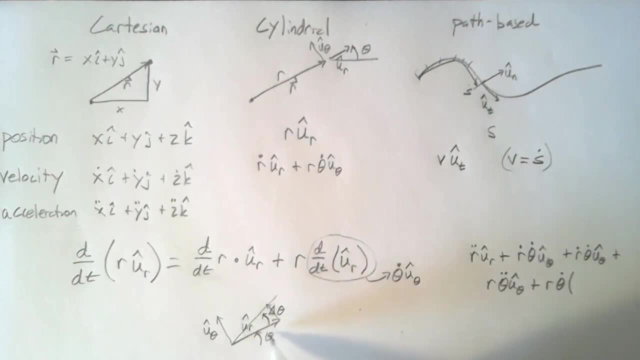 Well u theta is still defined by theta. So if theta's changing and moving all this around, we're saying that our delta theta is moving u theta in this direction. We're interested in seeing how u theta is changing And so our new u theta is in this direction. 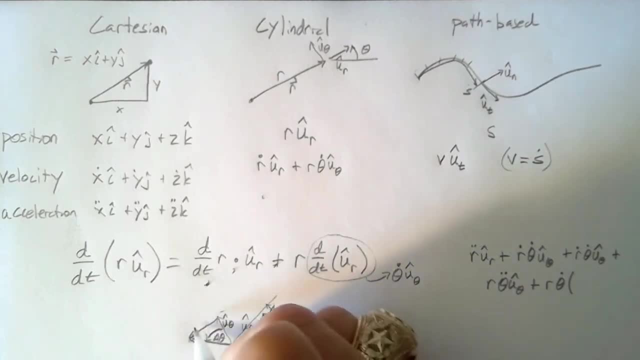 So we change based on theta dot multiplied by a negative u r. So just looking at the geometry, So what does this mean? over here, Now we have a negative theta dot u r. Okay. so let's clean this up a bit. 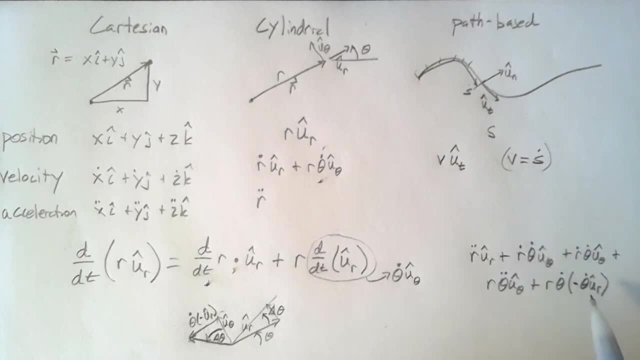 So we're collecting terms. now We want all the u? r terms, which are just these two, and all the u theta terms, which are these three together. So r double dot minus r theta dot, and we have two of those here. 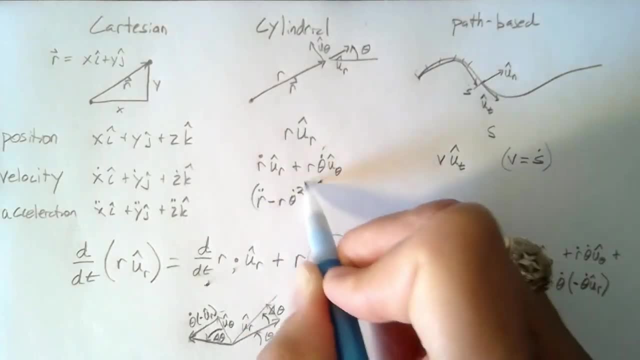 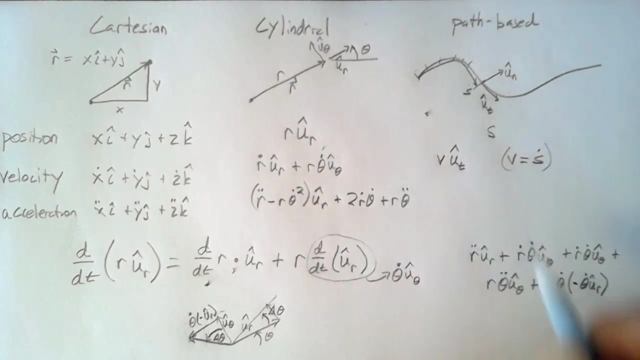 So this is actually r? theta dot squared, And all of that is in the? u? r direction. Okay, so now looking at the? u theta direction, u theta will have two r dot theta dot. Then we also have an r? theta double dot in the? u? theta direction. 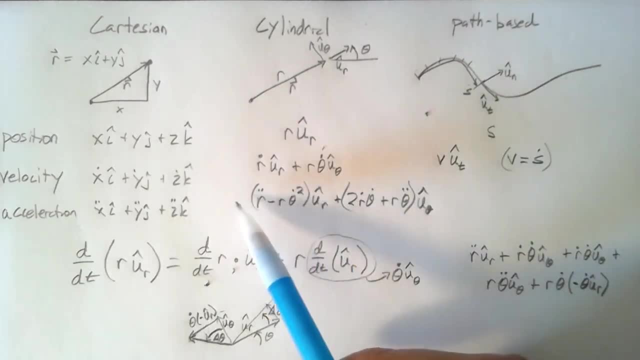 Okay, now let's look at these terms. We can get acceleration in the u? r direction based on some acceleration just directly outward. That's what this r? double dot term means. Now we can also get some acceleration because of just a change in theta. 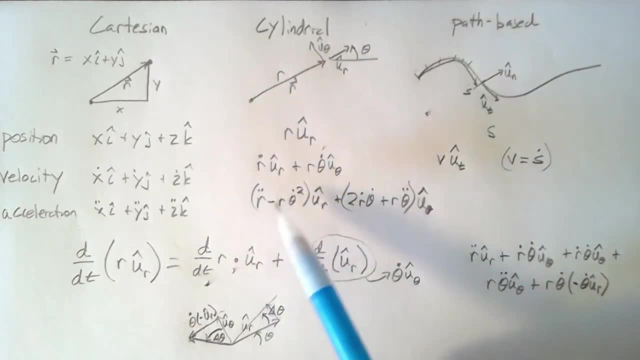 This is actually the centripetal acceleration, the acceleration seen by the particle because it's spinning. Okay, this one's also pretty easy. We can get some acceleration in this direction by speeding up how much we're rotating, So we speed up our rate of rotation. 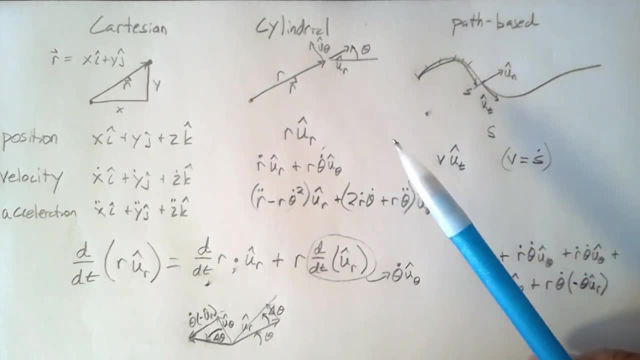 and then we end up with a acceleration pushing in the u theta direction. Now, this one- this term is probably the least easy to conceptualize- It's the Coriolis acceleration. We're going to hold this at a constant theta dot. 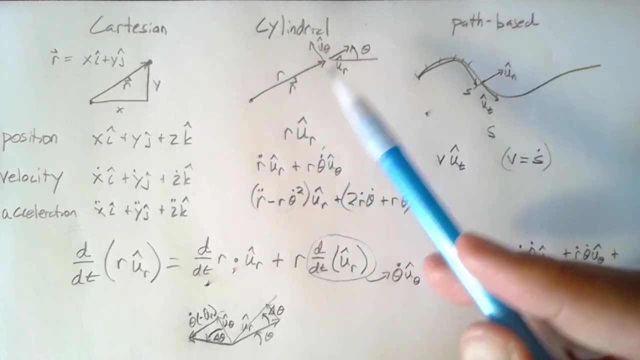 and then we're going to let this thing move outward. That requires us to accelerate in the u theta direction. Okay, once again, cylindrical required all of the math, and then with path-based, everything is just kind of plugged in to the definitions. 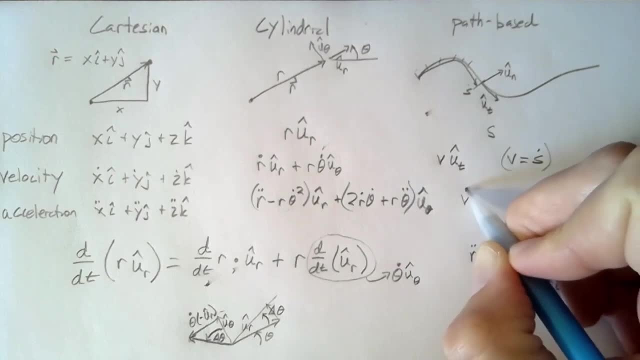 So we have some acceleration based on a change in the speed at which we're traversing this path, and that's going to be in the tangent direction. So our change of speed causes acceleration in the tangent direction, and then we need some acceleration in the normal direction. 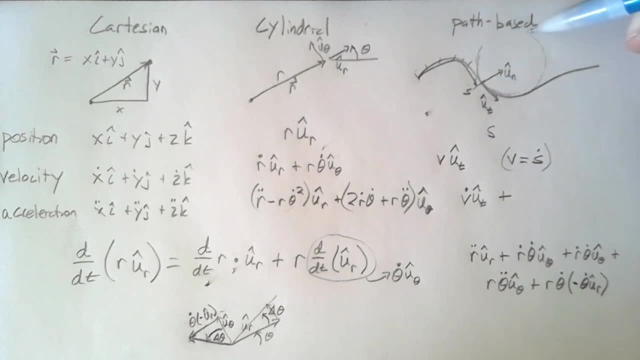 that's based on a radius of curvature. But we're going to look at this circle that encompasses our current point and say that it has some radius and we're going to call that radius rho. So, as this circle gets smaller and smaller, 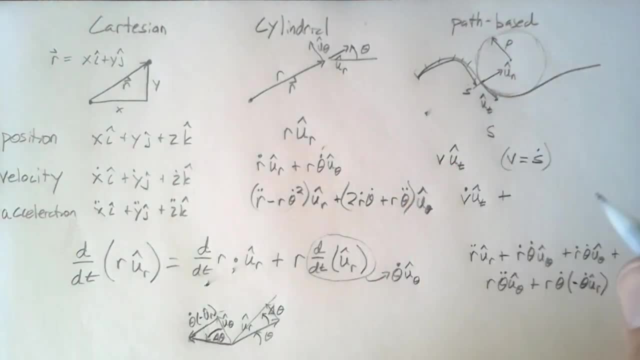 our acceleration needs to increase more and more. So this acceleration is v squared divided by rho in the normal direction. So as our velocity increases, we need more acceleration to keep up. We need more acceleration to keep on this path. And as this radius of curvature decreases,